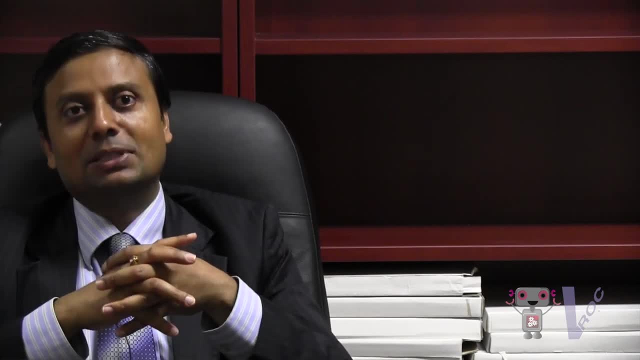 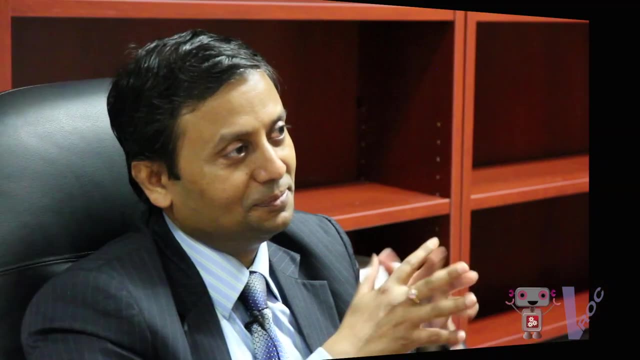 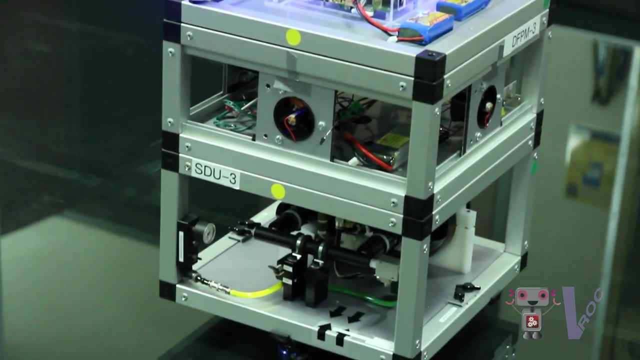 to you know, directly linked with the weight of the satellite. If the satellites weight lighter than it can, can directly reduce the cost of the launch. We have got the satellite design, complete design of the satellite. we do as well as we do the some of the components. 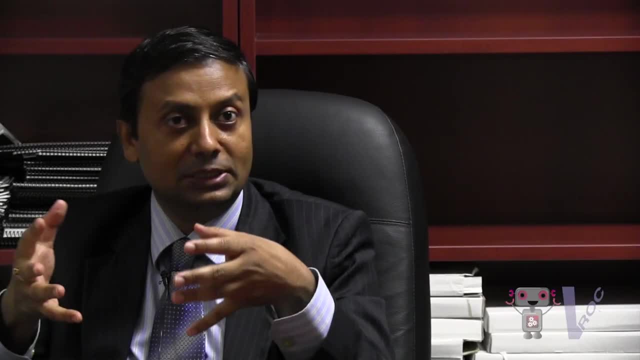 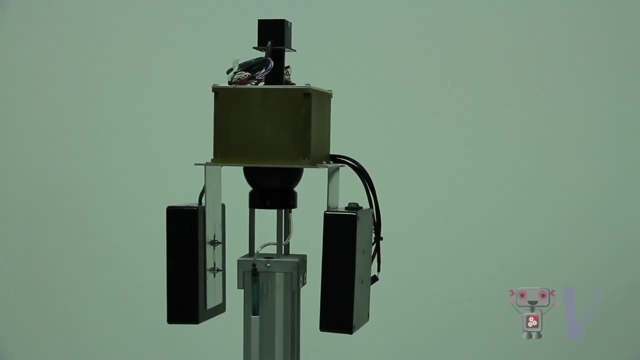 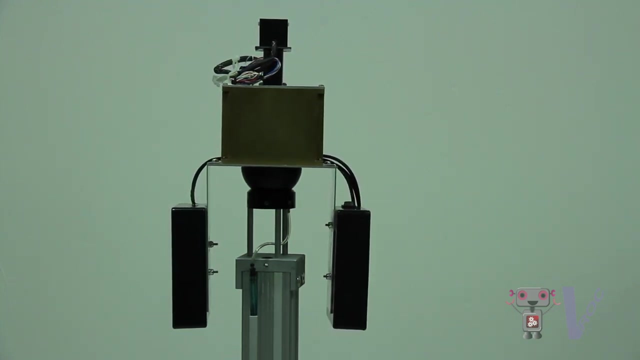 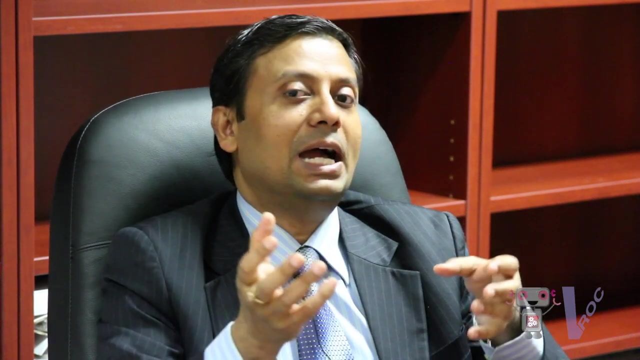 of the satellite. especially we do on attitude control system. Attitude control system means the device which control the orientation of the space. So we we have a system called reaction wheel that controls the attitude of the spacecraft. So we design reaction wheel system, We test on the ground to see that this, this can create. 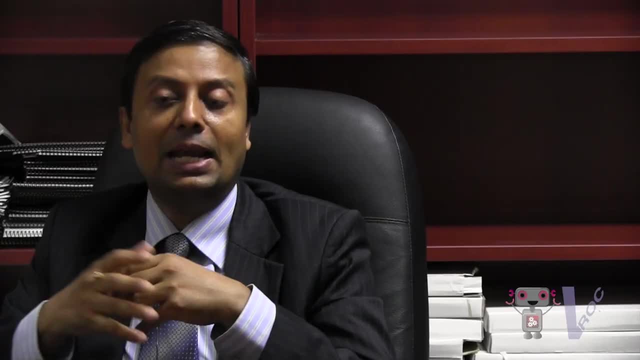 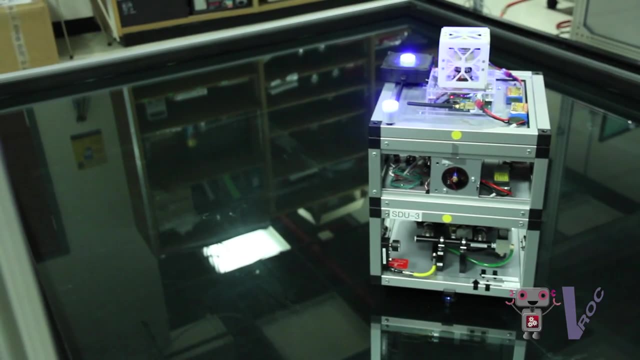 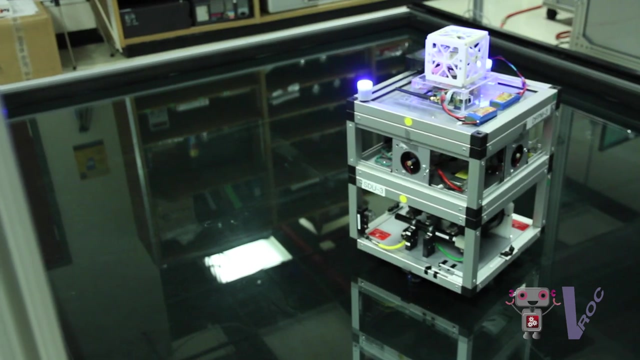 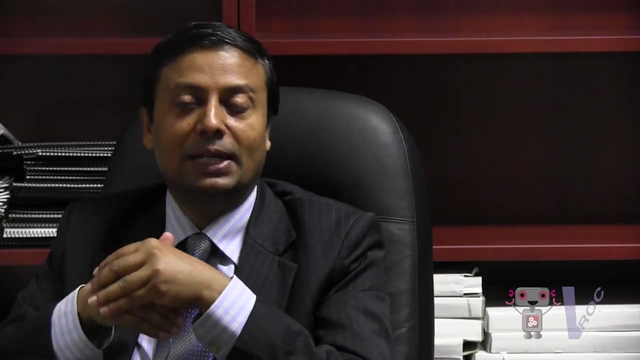 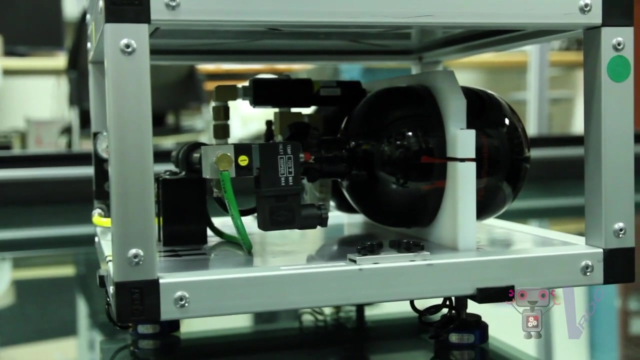 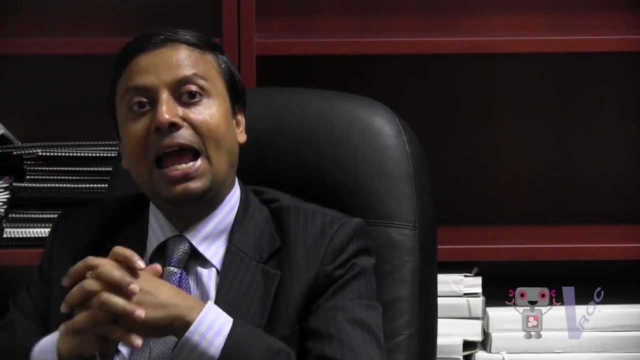 the satellite in proper direction, orientation And at the same time we have we also test how we move the satellite in the space. So we have got the formation test bed And we put these limits determined from preparations, we put a selection and 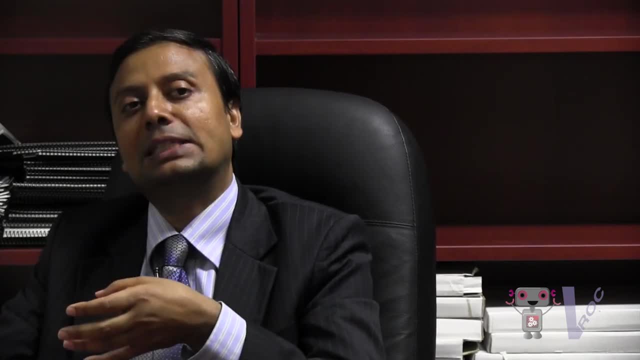 they are placed into the sat… In This, Yes, And then we have a control system, As now you have seen that in various ways they are has a alternating ah. instead they the satellite in the desired direction. 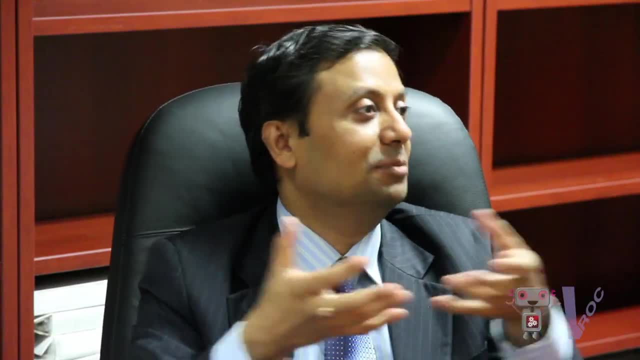 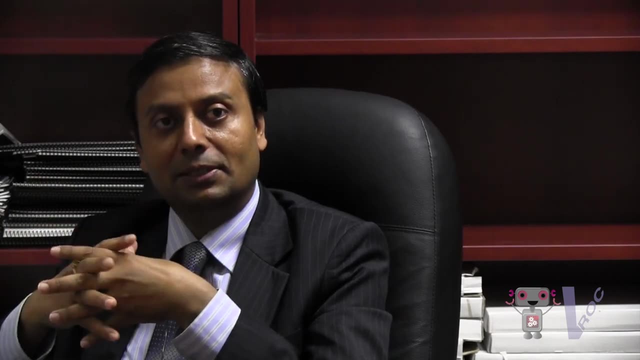 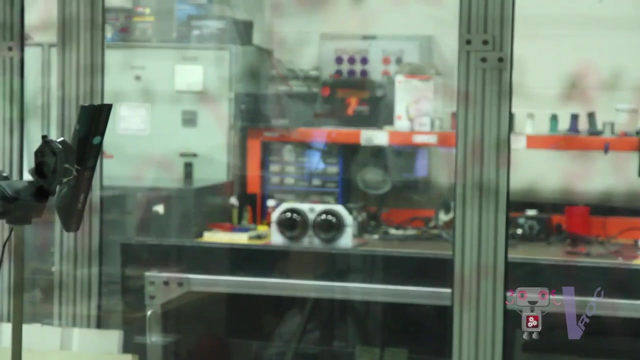 The design comes from the mission concepts. what is the application of the satellites, For example? if its application is to take image of the earth's surface, keeping that in view actually, then we try to design different subsystems of the satellite. First of all, he should definitely have very strong by-ground in mathematics. that's a. 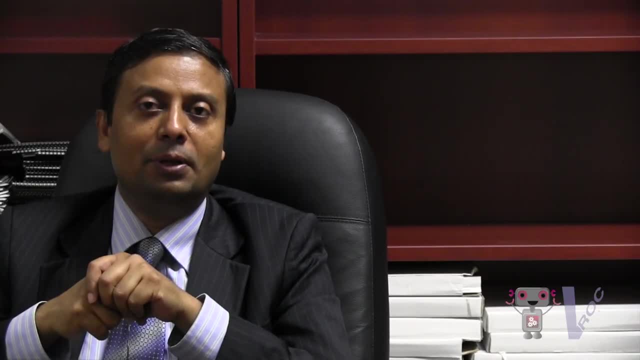 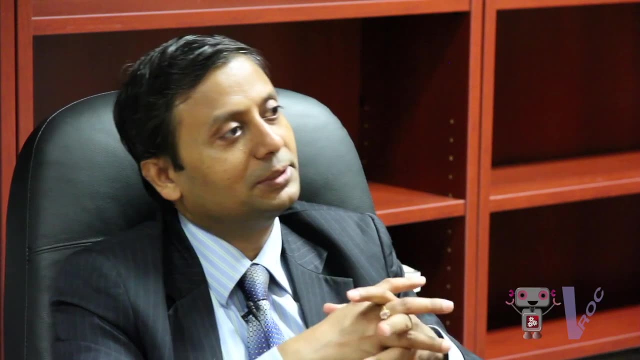 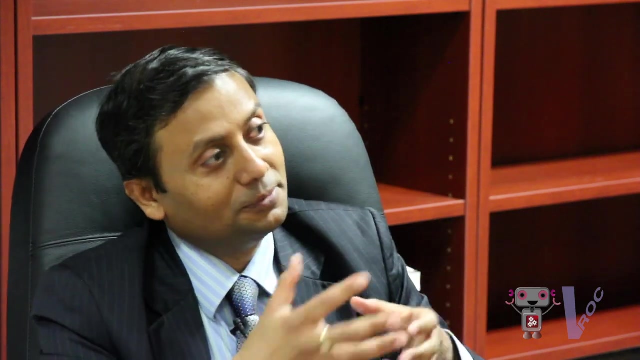 must, Then he should have a strong by-ground on designing the system. Design means using some software, like we have a SOLIDWORKS, so how you can construct it. Also, he should have ability right. this design can be manufactured in a machine. 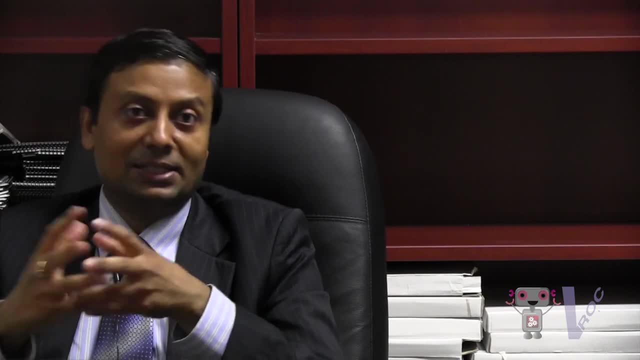 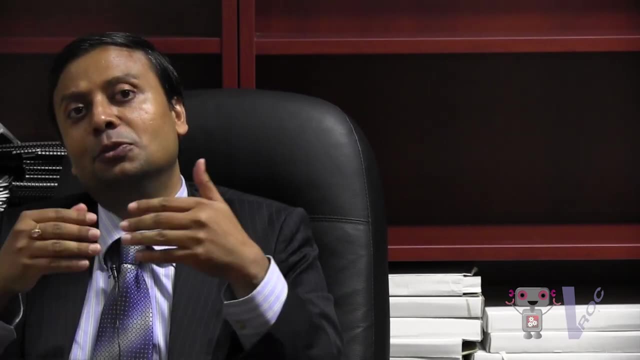 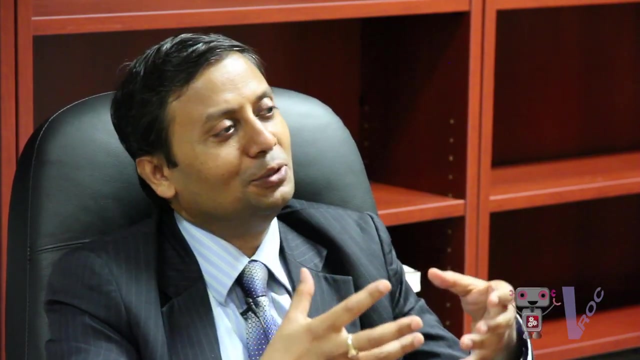 And at the same time he should have a by-ground on electronics circuits so that he can build the satellite. They should be motivated to pursue a career in aerospace and they should have a passion. they want to really, You know, do work in aerospace industries.